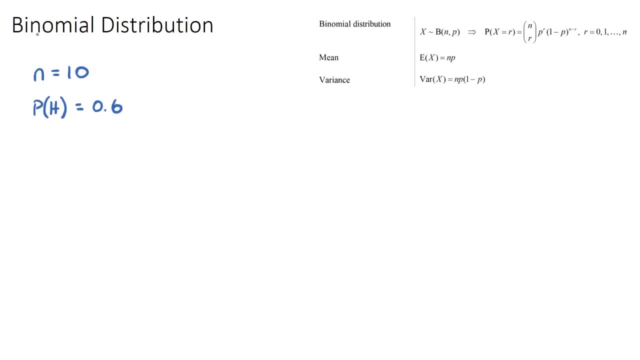 will just be one minus this. So binomial distribution questions, they're not going to be a bunch of different probabilities. It'll just be a success and then a failure, And if we know the success probability, the failure will be a success. 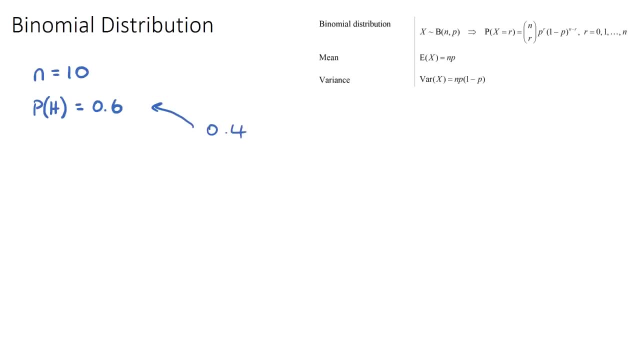 The failure will just be one minus that, which will be, in this example, 0.4.. Okay, so heads will be a success for this question, And once we know the number of trials and the probability of success, we can solve a bunch of questions. So what's typically asked? 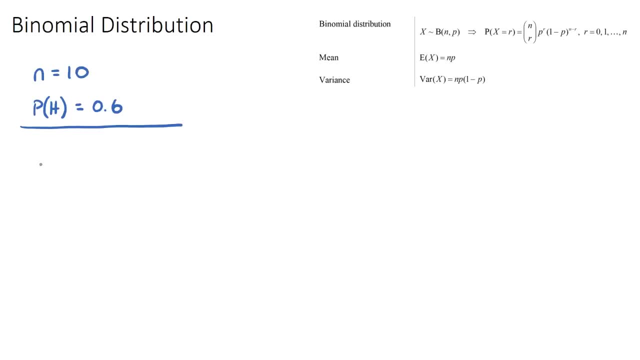 after this is they'll say: well, what's the probability that the number of heads that we get- So let's just say a random variable- is how many heads we'll get in the 10 flips. What's the probability? this is equal to three. So you might think, oh okay, that could happen. a bunch of. 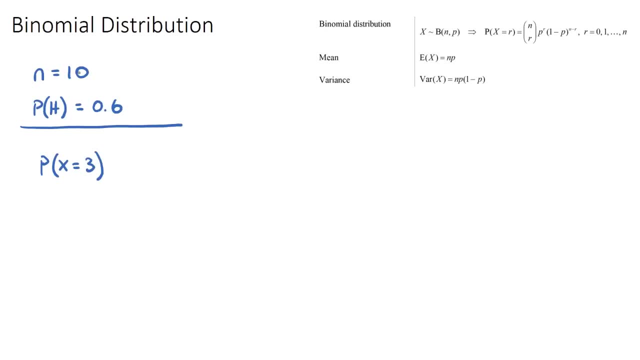 different ways. We could get three heads early on and then seven tails, Or we could get three heads at the end and then seven tails at the start. Well, there's actually a lot of different ways, And the mathematical way of finding the formula to find this answer is actually quite complicated. 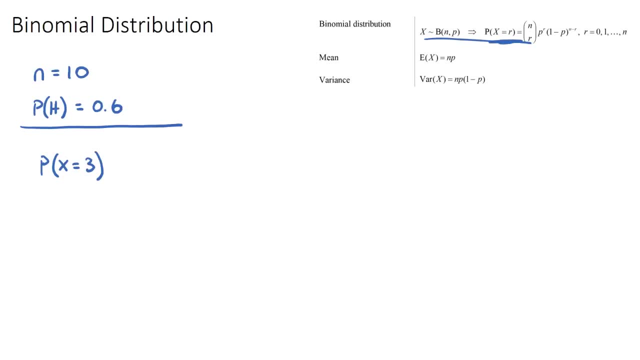 And it's this one up here And, lucky for us, our calculator does do a lot of this work for us, So I'm going to show you how to find this answer. And I'm going to show you how to find this answer. 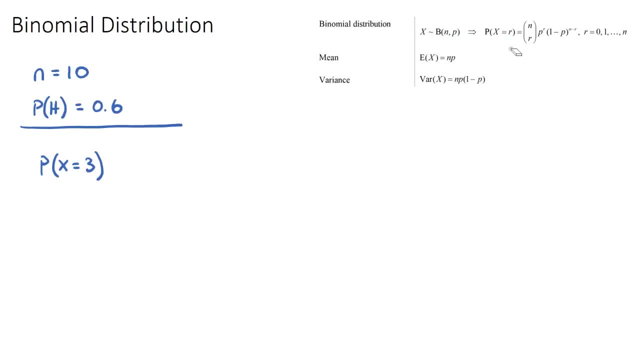 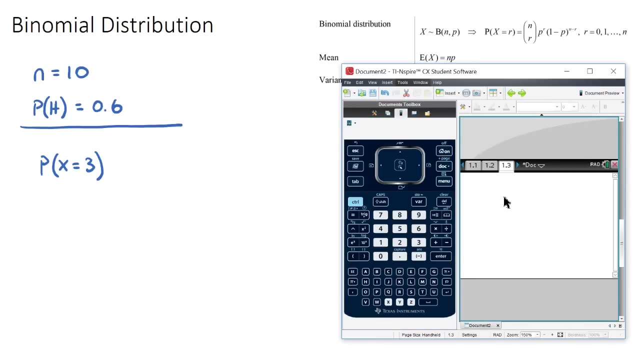 how to do it on your calculator and then I'll refer back to the formula to see where we got these numbers from. So we want to go to our calculator. Now. you can just open up a new calculator section and if you go to menu probability, you want to find your distribution. 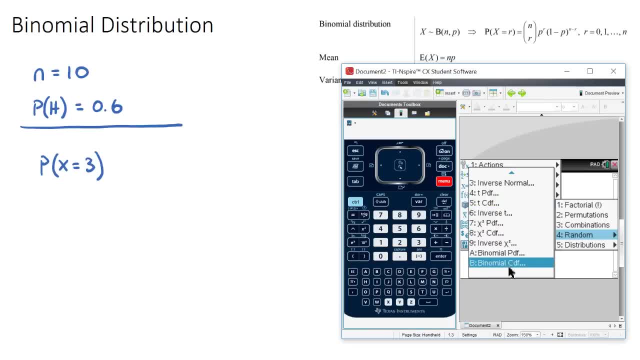 section of your calculator and this is a binomial question and we're either going to be using binomial PDF or CDF. Now we use binomial PDF when we want to find the probability of getting an exact amount of heads or whatever variable you want. So in this case, we want exactly three. 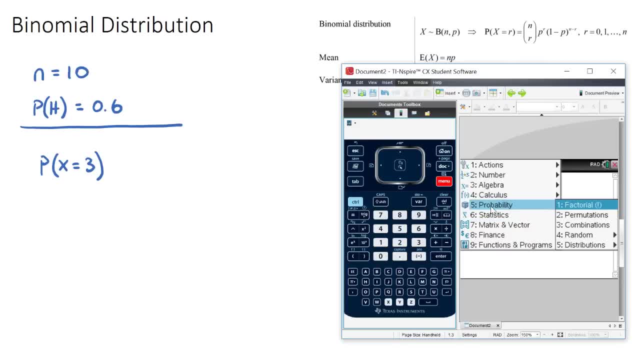 and if it's the exact number, we want to use binomial PDF. So let's use PDF. It asks us for the number of trials, which is 10, the probability of success- Now, success here would be getting a head- and the probability of success. we want this to happen three times and this will give us the. 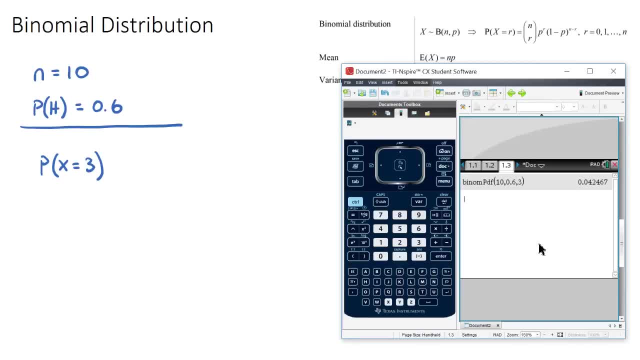 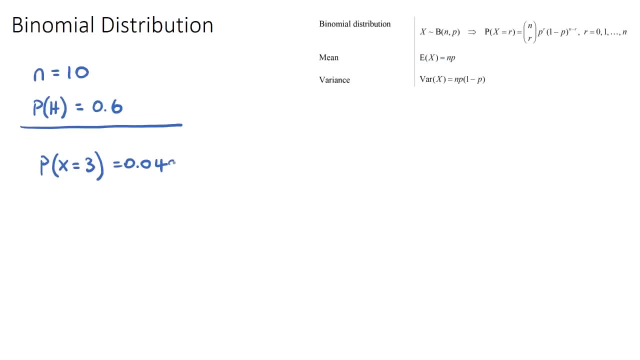 answer: 0.0425.. 0.0425.. Now, if you're very interested in how this formula appeared, what actually is happening is we could get three heads out of 10 in 10c3 ways. This is the combinations. 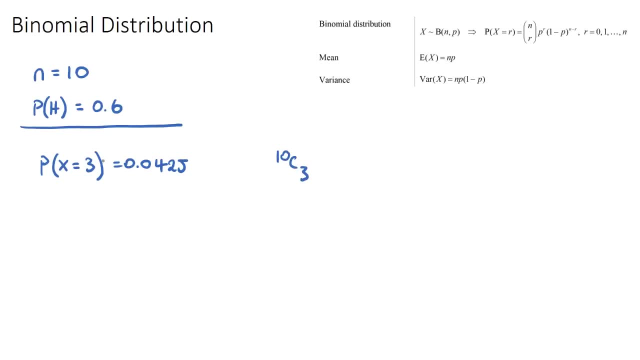 component of this formula. and then a head has a probability of zero, 0.6, and we know we had three of these, so 0.6 and 0.6, and 0.6 to the power of three, and then it would be tails 0.4 to the power of, and there was seven of them. and then this is the complex formula. 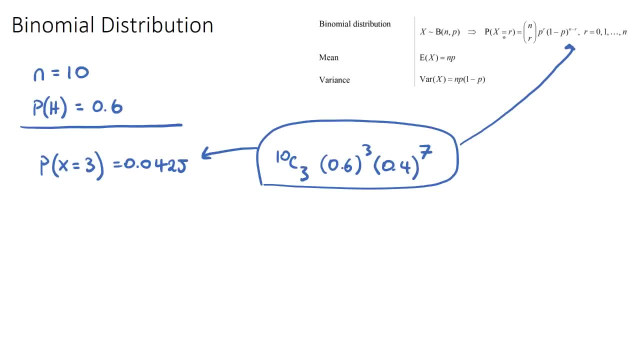 which got us this answer, and that's what this is actually saying up here: The probability that our random variable is r, which is n, the number of trials, cr, the probability of success to the r, and then the other probability, 0.6 to the n minus r. So this is quite a complex formula, but if we use the calculator and you use 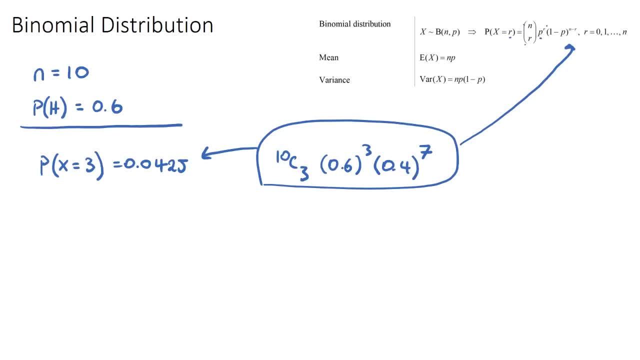 the binomial PDF, it will solve it for us. Okay, so if we said the probability that x is equal to, let's say, seven, we can use our calculator again and what we're going to get is probably a higher probability. because if we, if we have a probability of getting a head as 0.6 and we have 10 trials, 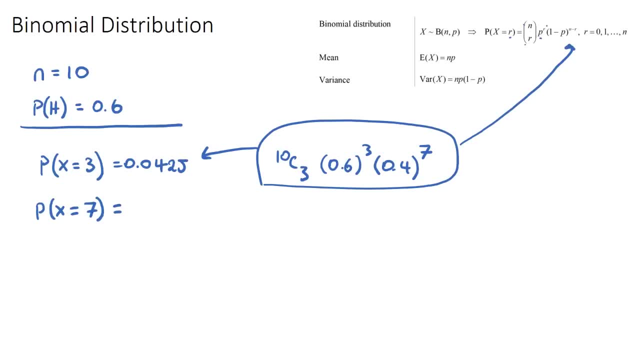 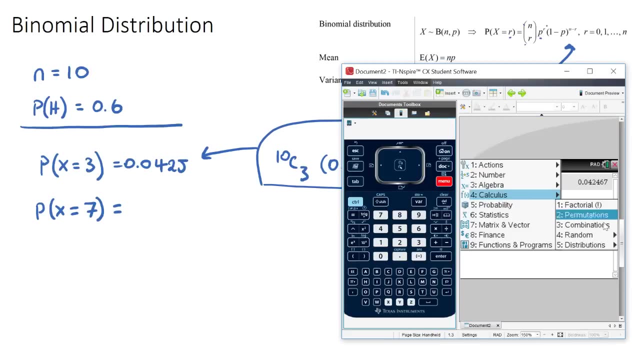 three was. getting three heads would be pretty unlucky, but getting seven would be more likely. So if we were to do the same step, I would assume we'd get a slightly higher probability. Let's go to distributions binomial PDF. we have 10, 0.6 and we have seven and we have 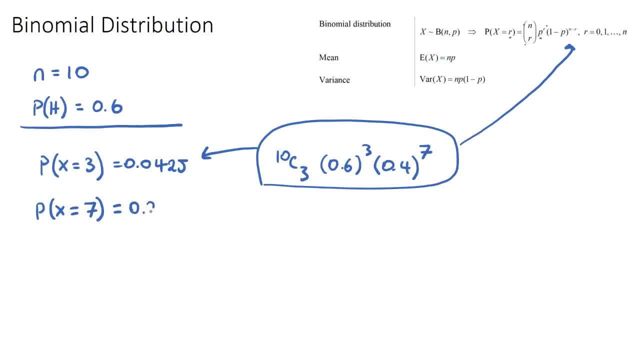 0.215, this time 0.215.. Okay, now if they asked for: well, what's the probability? you get three or more heads. So x is now greater than or equal to three. So that means we could get three heads or four. 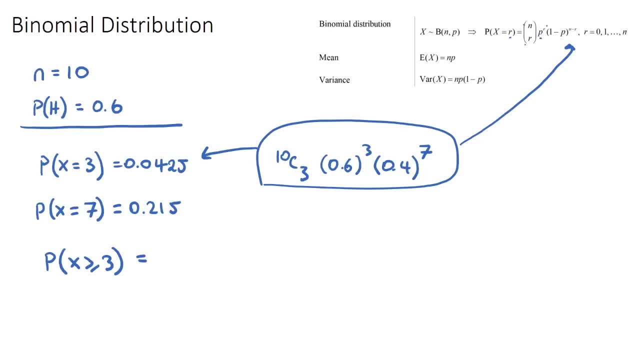 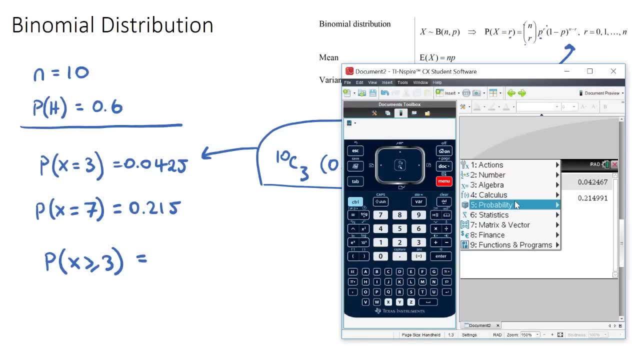 heads, or five all the way up to ten heads out of the ten trials. And if we have a group of scores we use binomial CDF. So we go and find the one below it in distributions and CDF has the lower bound and upper bound, So the number of trials will still be ten. 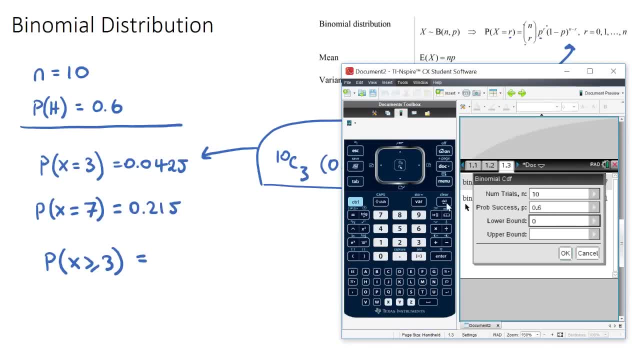 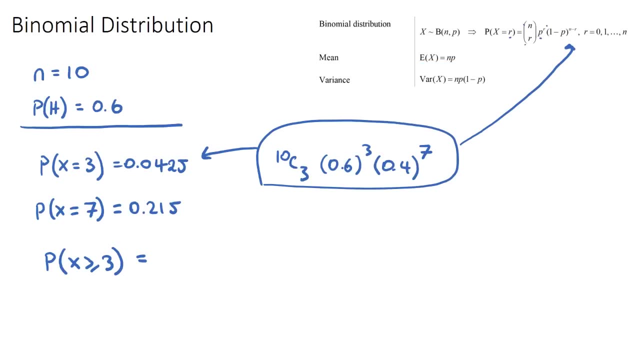 We'll have 0.6 and the lower bound we want three or more. So we'd have three and the upper bound would be ten out of ten heads, And this is very likely, very likely. So we'll get a probability of 0.988, 0.988.. So that's what that's when we use binomial PDF and CDF. PDF finds a particular. 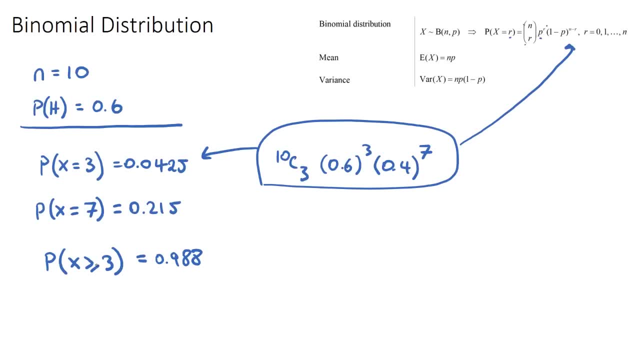 number of heads We want to get, and CDF is a group of numbers that we want to get. And the other two formulas that you see here, the mean and the variance. these are pretty simple formulas, these ones. What this mean is a mean is the same as the expected value, And that just says that. well, if we do ten trials and 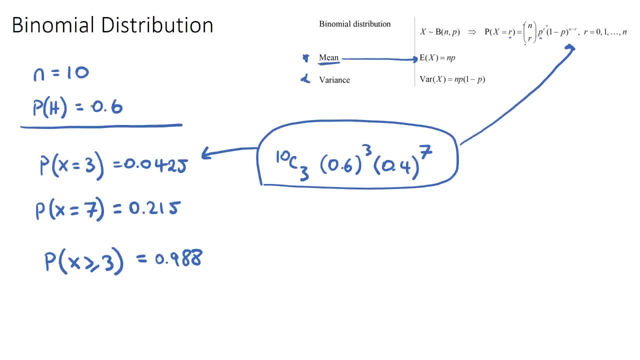 each trial has a probability of 0.6, how many are we expected to get? And then that formula, I think, makes sense: It would just be ten times the probability of 0.6.. So that's what that means: If we find 0.6, which would be six, and we would expect to get six heads if we flipped it ten times. 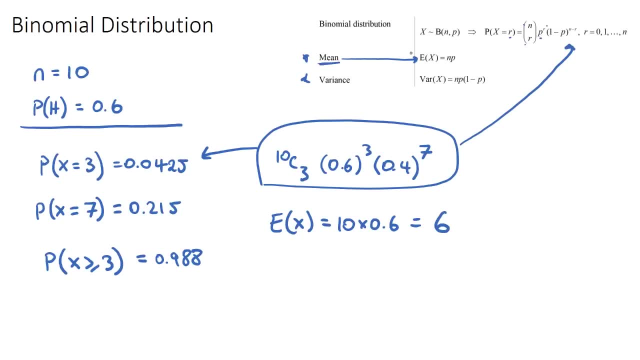 and the probability was 0.6.. So this formula: the question will ask for the expected value or the mean, and it just means we multiply the number of trials by the probability. And then some questions. these are a little. these aren't as common, they're a little bit more rare. but if it asks for the 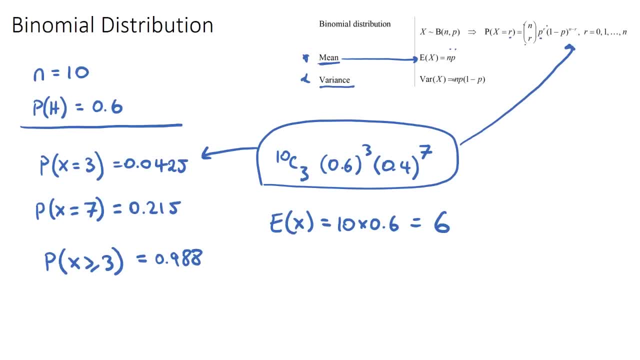 variance of a binomial distribution question. it's just the same formula as above, but we need to multiply our n and p by the other probability, the failure probability, So it'll be np. so our variance will be 10 times 0.6, times 0.4, the opposite probability to the success, And we can.